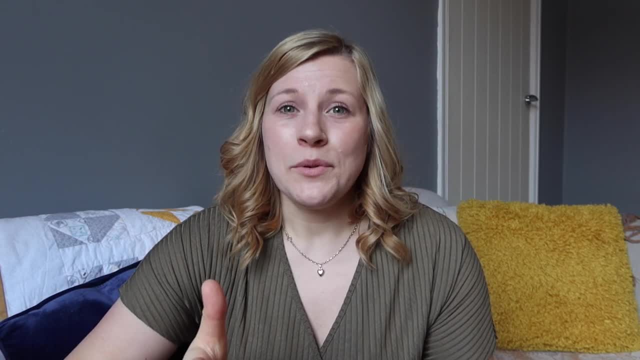 to wear, then this is a great option. So if you do have a toddler and you're looking to get a little creative and find them something to wear, then this is a great alternative. It is simple to put together. It does require a few more parts than just a simple pattern. So if you are looking for 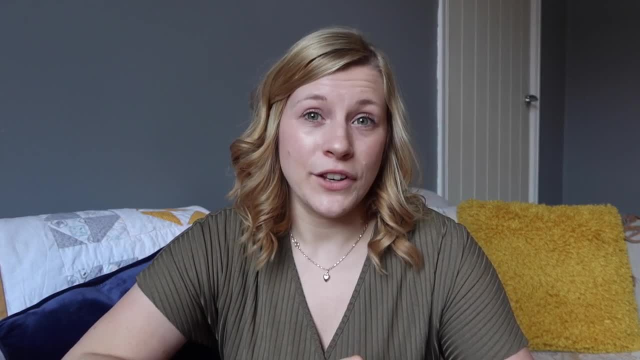 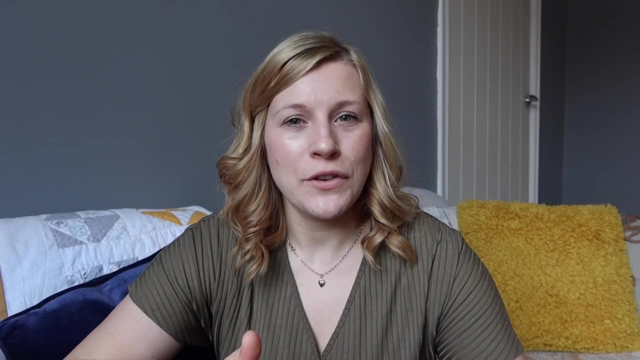 something a bit more complex, a little bit more challenging. this is definitely the pattern for you. Number two on the list is a baby t-shirt by Melly Sewers. If you don't know Melly Sewers, then this blog is perfect for you. It's got so much comprehensive information about getting started. 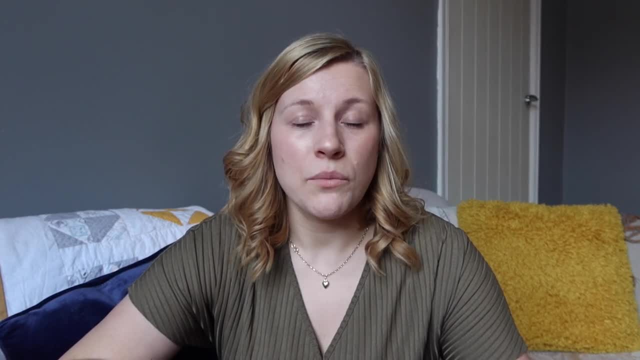 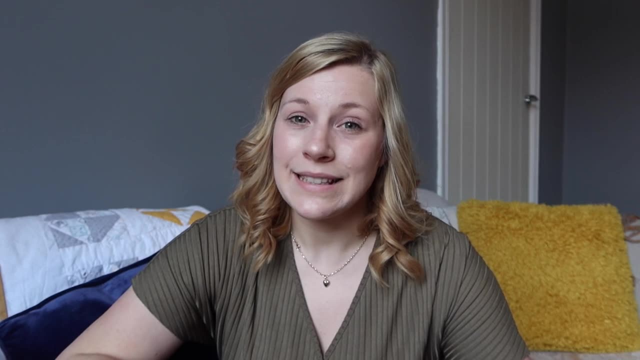 with sewing cloth making, So if you are looking for more hints and tips, then go check that out. We're going to talk about the pattern, which is really simple and really easy to follow. You can use an old t-shirt of your own to create this, which I love. You don't have to go out and buy. 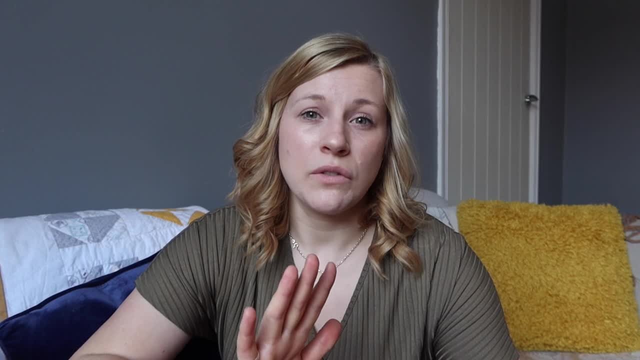 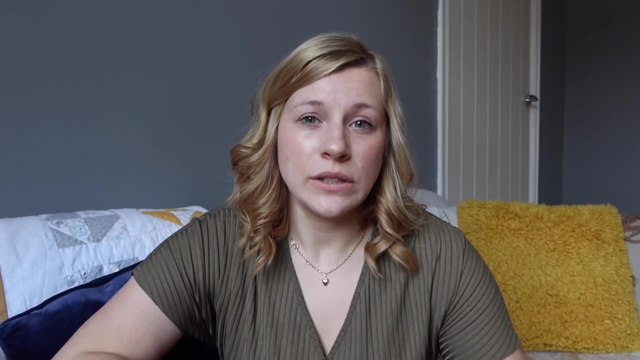 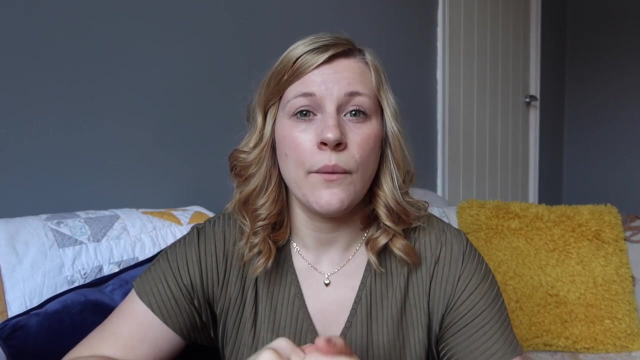 any speciality fabrics. Just make sure it's washed and there's no real big stains on it and you can cut out the pieces just like that. So this pattern comes with one size only. I'll put the link to the pattern. I'll put a link in the description below so you can go check it out. 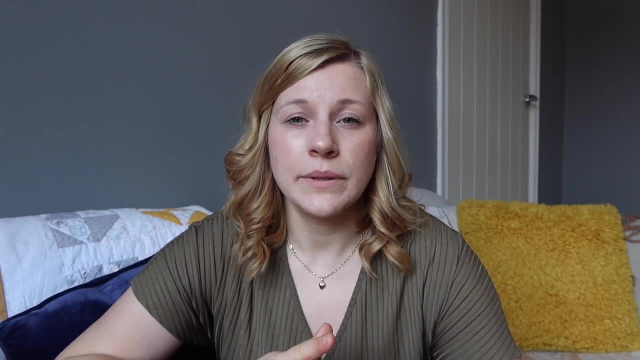 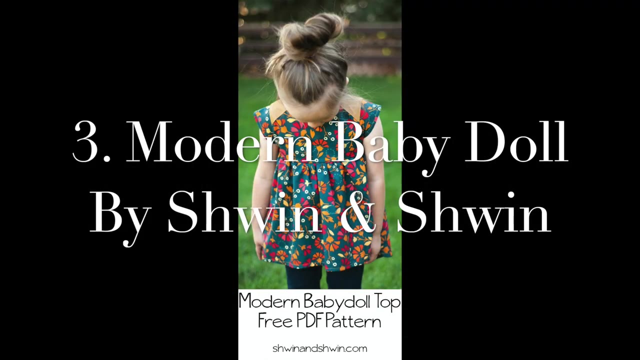 but you can use that then maybe to upgrade it Or make it a little bit smaller if you, if you feel confident. If not, there's plenty more on this list for you. So number three on the list is a modern baby doll dress by Schwinn, and Schwinn I quite 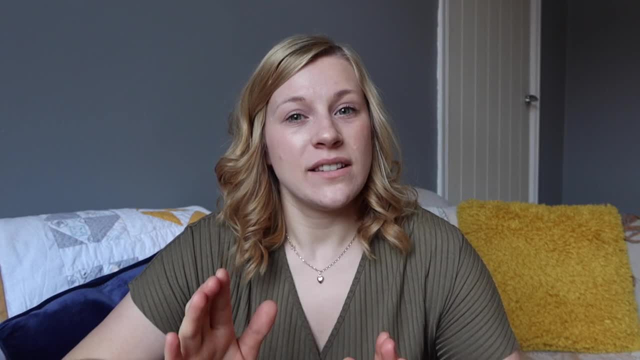 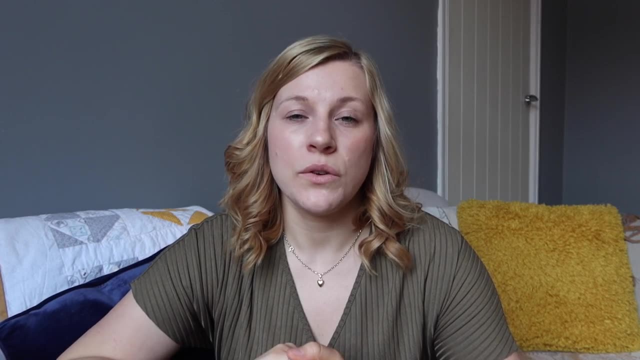 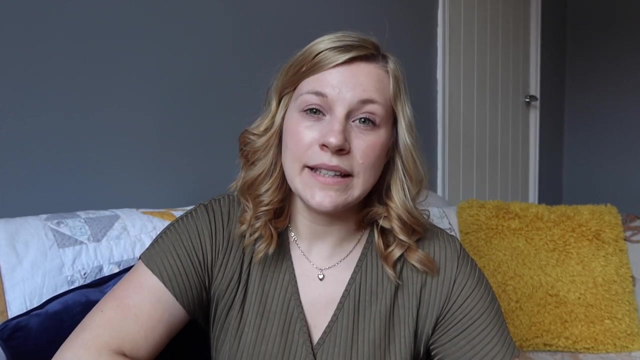 like that name, And this is for the ages five to six only. Again, there is an alternative pattern for older years. They'll have that within the blog post, so if you want to purchase that, then you can do, But this is the free version for five to six years. So this is a really fun and 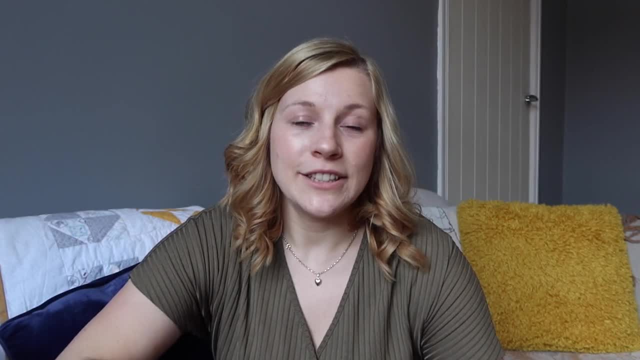 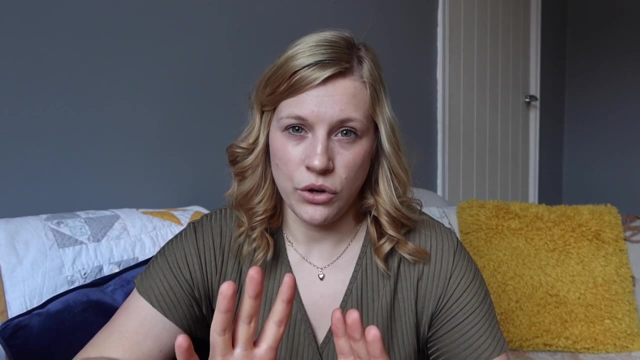 creative pattern Perfect for making a little. you know, dress for summer Does come with a zip in the back. so if you are still in the beginner stages and not quite wanting to conquer a zip, then maybe pass up on this one and go back to it at a later date when you feel a bit more confident. 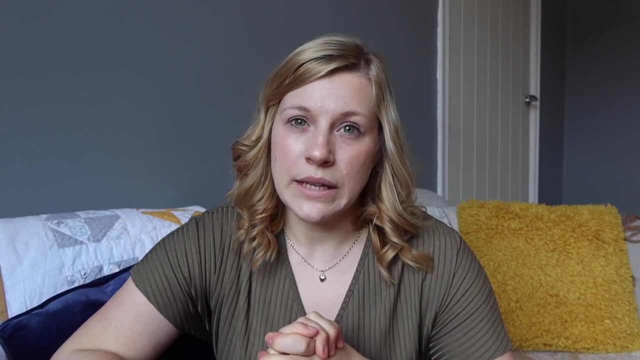 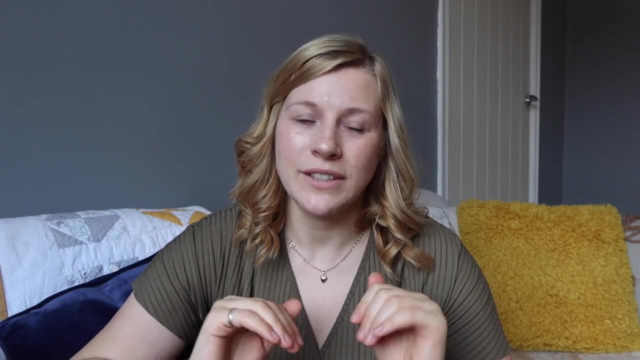 and have tackled zips. I still struggle with zips. No shame whatsoever. If you can't do them, just move on for now. Come back when you feel a little bit more confident. So number four on the list is a basic kids dress. 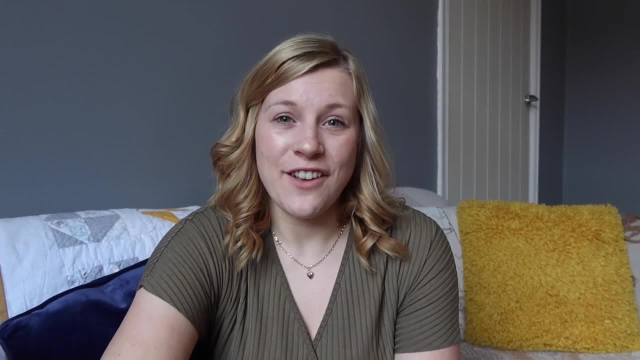 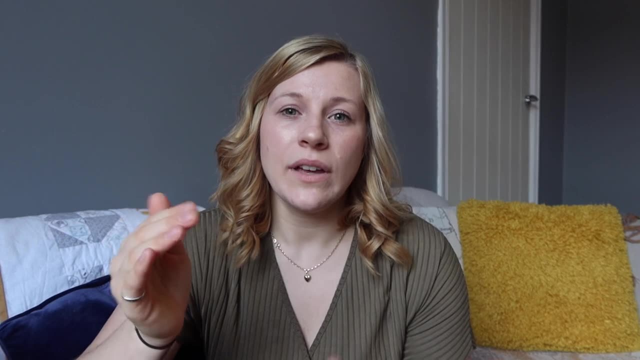 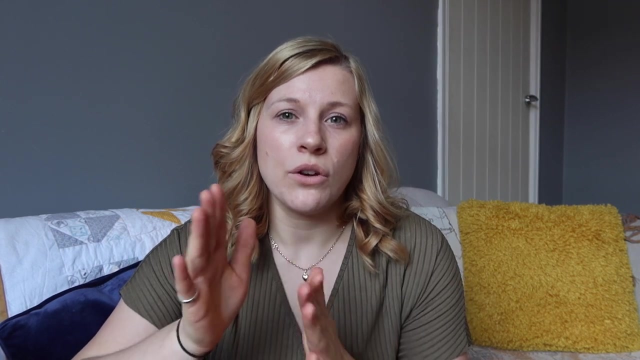 This is made by Everyday with Darna. The sizes are 2T to 3T, so that is an American size. I'll leave a link in the description or a kind of table with like a conversion chart from UK, Europe and American sizes and where that sticks. So if you're unsure of the sizing, then I'll you. 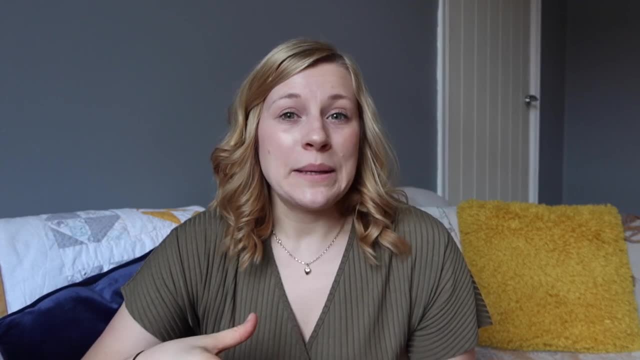 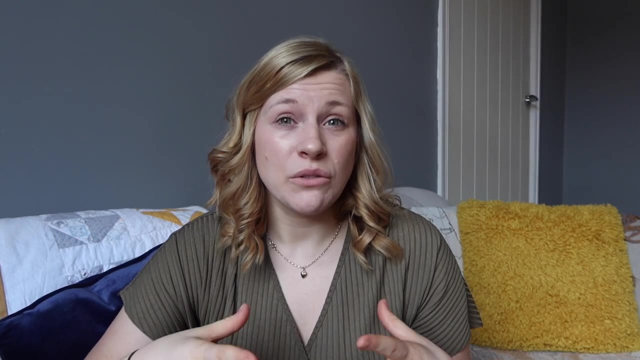 know I'll leave the information for you below. So I love this pattern because it's really simple and you can use it to create shorts If you want to make a little bit more of a dress. So if you're wondering if you want it as well or, you know, make them into formal trousers. you can use these to. 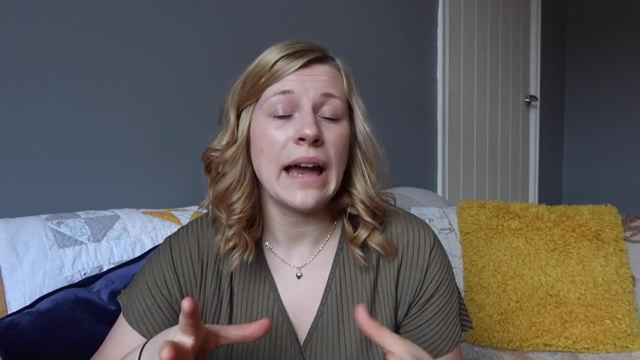 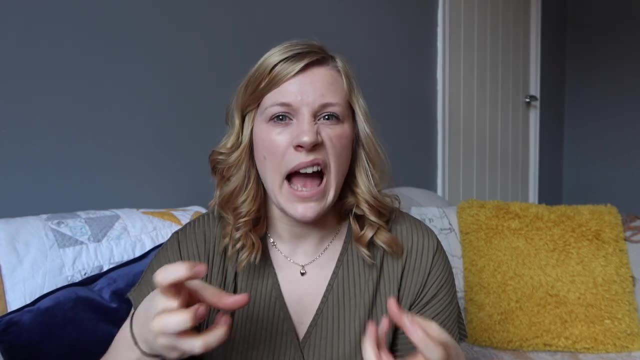 make them into joggers, You know. cuff the hem, You know- there's all kinds of different things you can use this basic pattern to create, especially if you are quite- you know you quite like hacking a pattern, like I do, Making it something new and really getting the use out of a pattern. This is one of 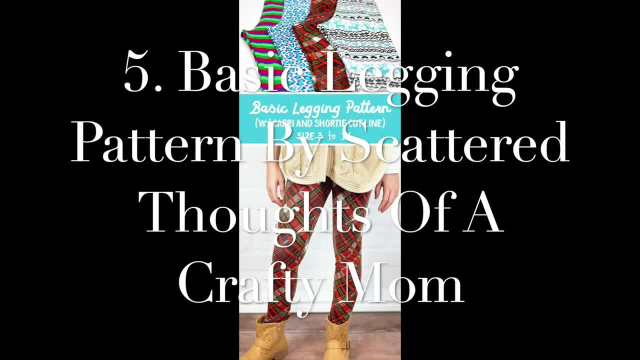 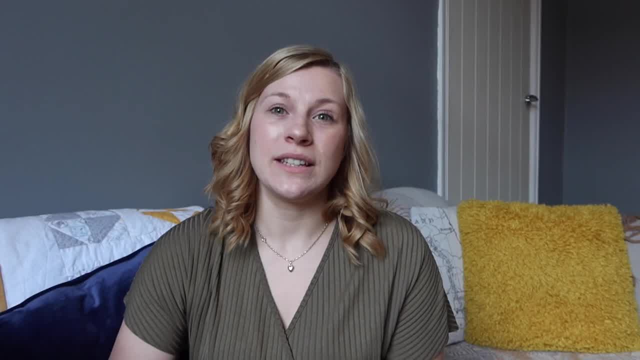 those patterns for you. So number five on the list is a basic legging pattern. So this is ages 3 to 14. by Scattered Thoughts of a Crafty Mom. This pattern is perfect for anyone who's looking to create some leggings for their children. 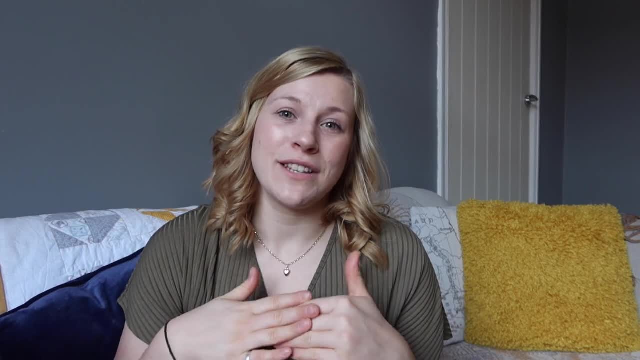 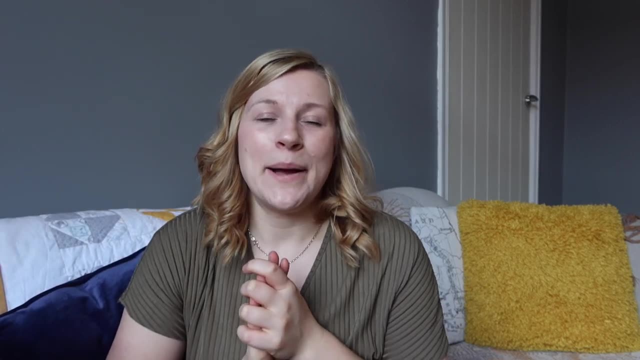 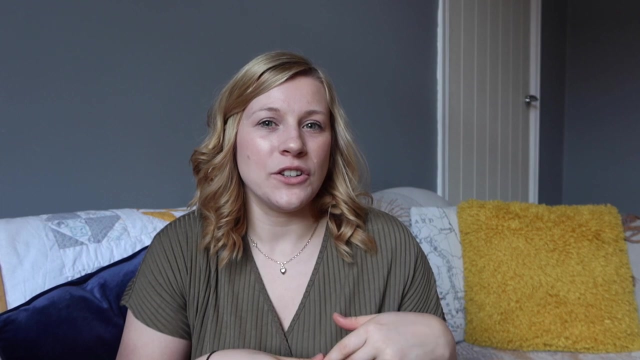 Thewhat I like the most is it is from ages 3 to 14, so you can keep using this pattern throughout the yeartheir age range, And it's just perfect because you can use this to hack into like little cycling shorts and you can add these. you know, you can make them little shorts to put. 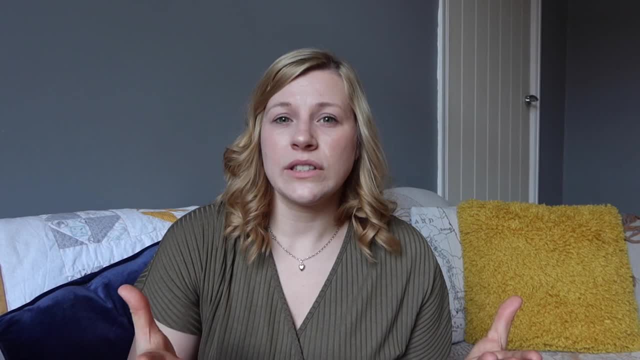 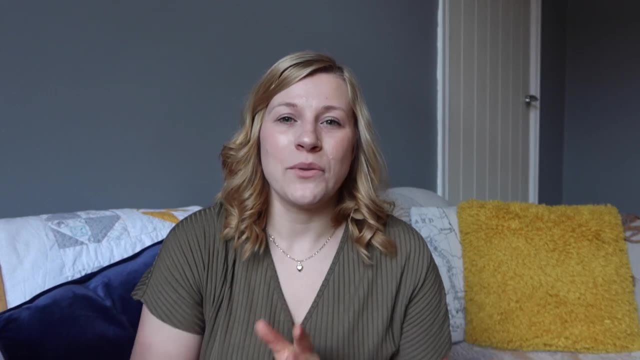 under their skirts. So if they're when they're at school, or even you know when they're out and they're running around And you don't want, wanted to see their underwear, so a little pair of shorts underneath is nice, just to give them coverage while they do the cartwheels in summer, and it's just. 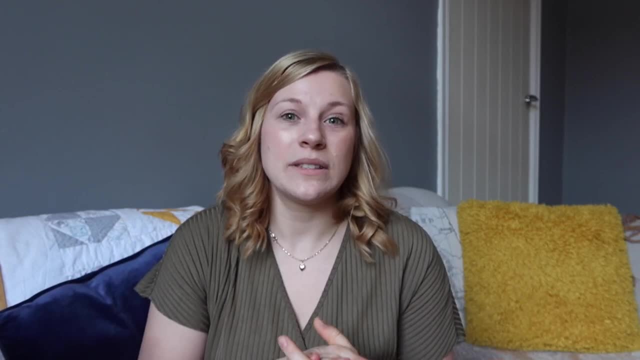 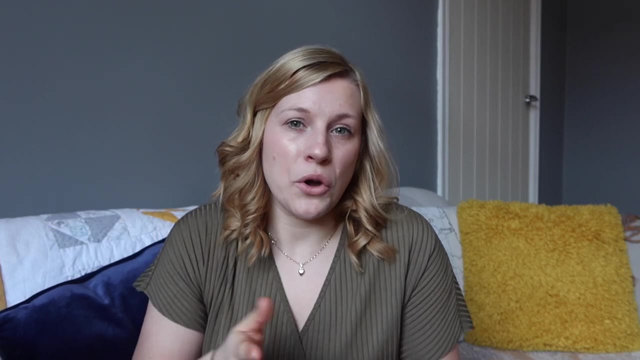 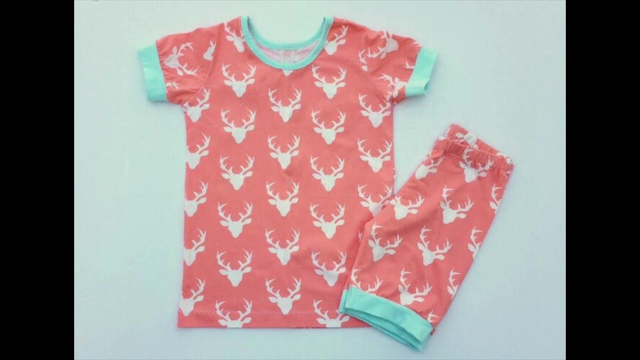 really fun, really easy to put together and you can use again t-shirts that you've got a home and or, you know, fabric that you found in your stash, or go and buy some new ones purposely. number six is a short sleeve pajama pattern by DIY crush. this is perfect for if you're wanting to make those matching pajamas. 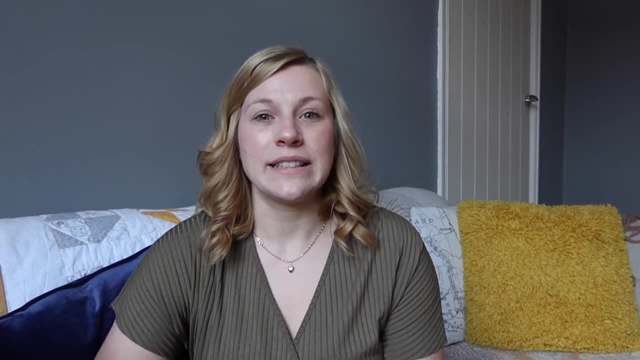 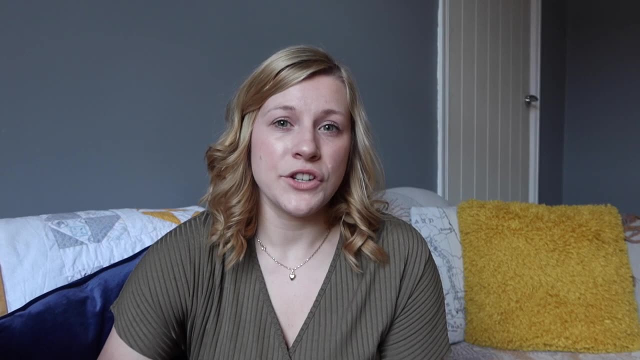 at Christmastime, which everybody loves, or if you're just looking to spruce up your kids wardrobe with some nice comfy pajamas. what I love about this pattern is you can use it for all kinds of ages, and both boys and girls. it's not gender. 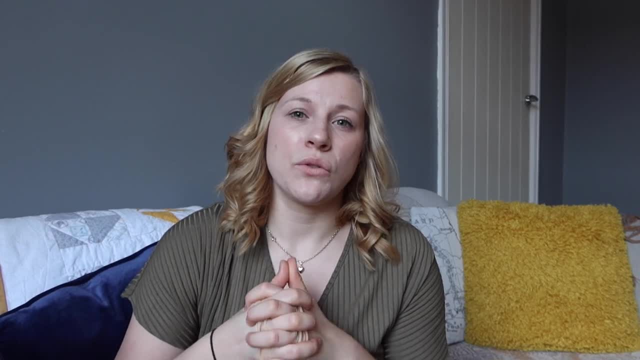 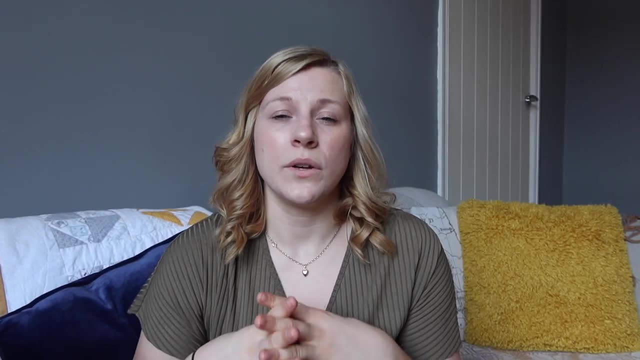 specific. so this is great because you can use this across the board for a number of children. especially if you have both boys and girls within your household. finding a pattern that works for both is blessing, because then at least you know well that one pattern it works. it will last for a long time. 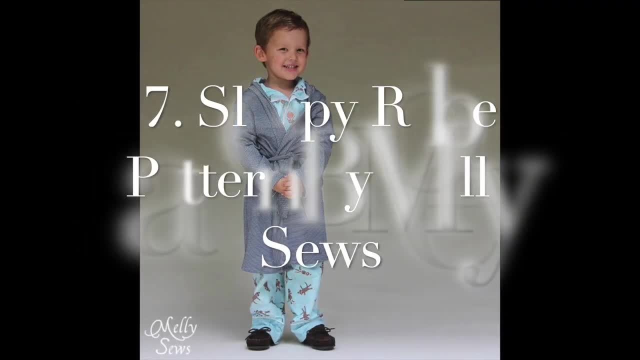 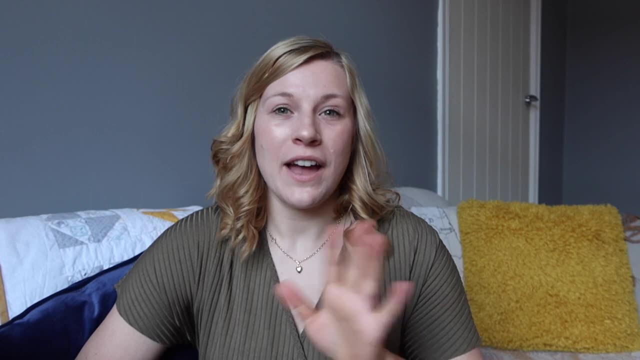 it will work for the other children as well. so number seven on the list is a sleepy robe pattern by Milly soars. what I love about this pattern is it again is unisex, so you can use it for any children you've got, whether it's nieces. 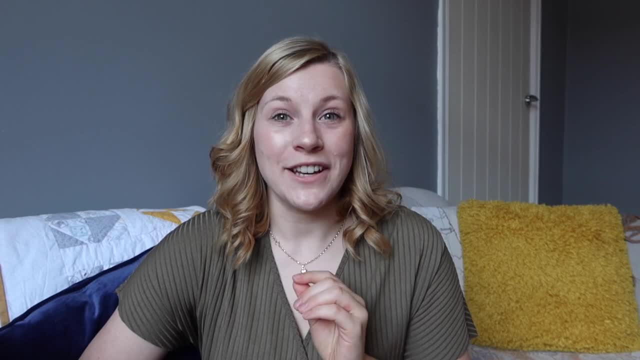 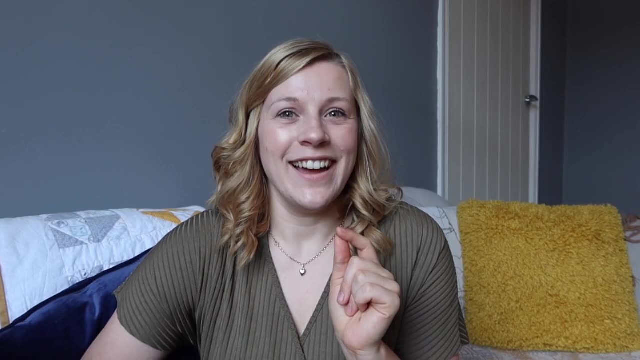 nephews or your own children. it also comes in a range of sizes, perfect for if you are wanting to create little matching robes between the children. just love that idea and this. so this is really simple, really basic to put together. everything is suggested for you, what you. 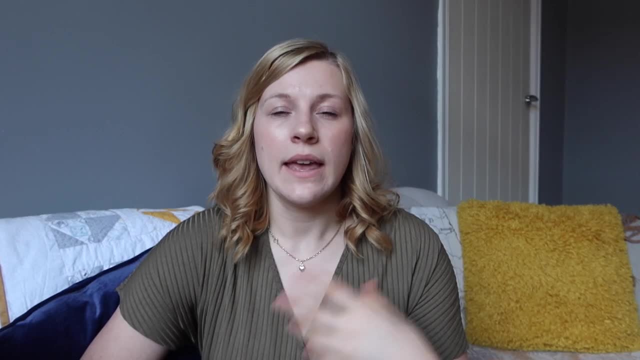 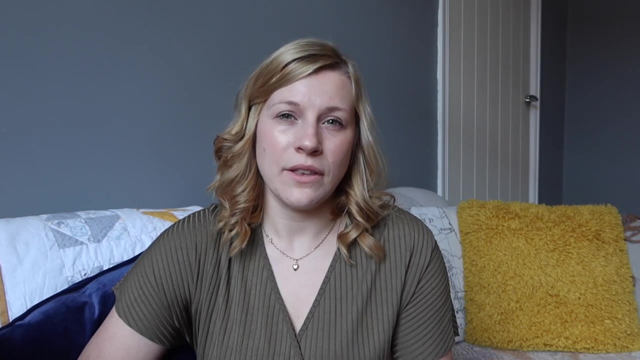 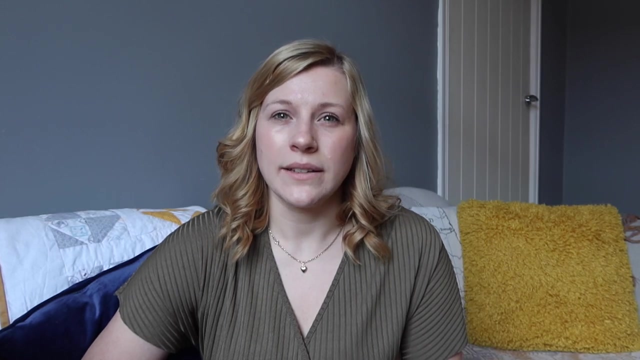 know the materials you'll need, how much you'll need of everything. any extras such as fastenings or linings or anything like that will be suggested, and the the whole tutorial throughout is so simple to follow and so basic. it's a great beginner pattern as well to use if you are looking to try out your first. 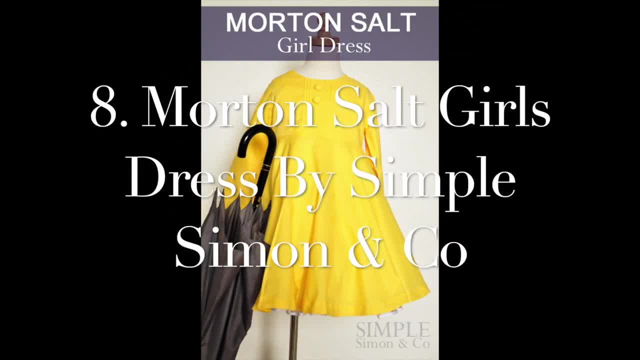 clothing pattern. so number eight is the Morton salt girls dress by simple Simon and Co. I fell in love with this as soon as I saw it. it was so good. I'm going to show you how to make this pattern and I'm going to show you how to make this. 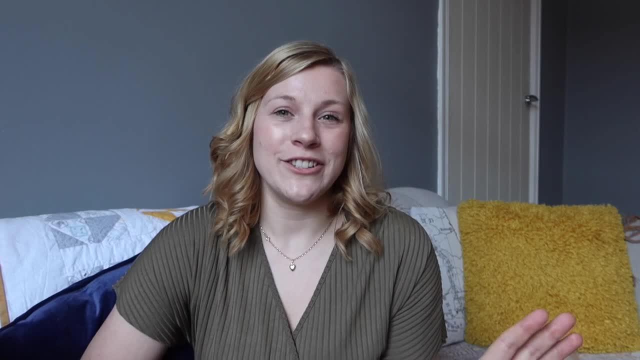 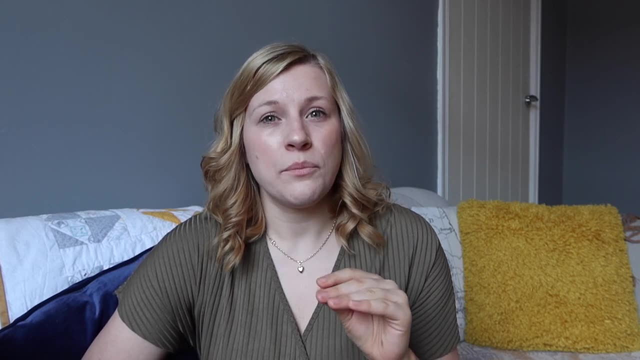 simple Simon and Co. I fell in love with this as soon as I saw it. it was so cute and I've already downloaded it ready to make for my niece because it's adorable. it is a restricted size, just to age five, but I think there is a link to 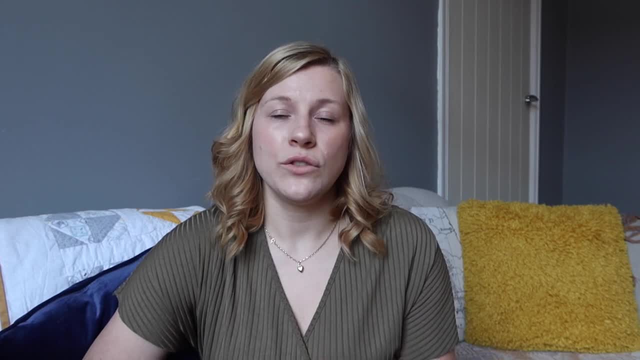 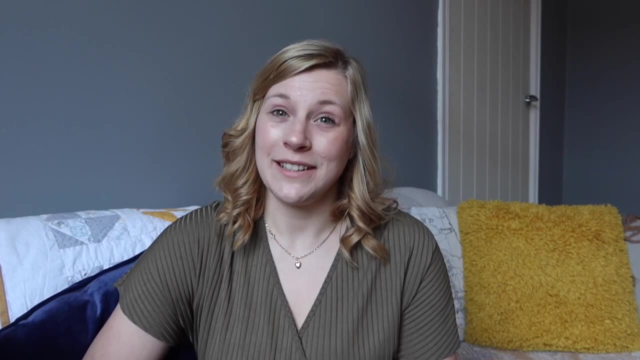 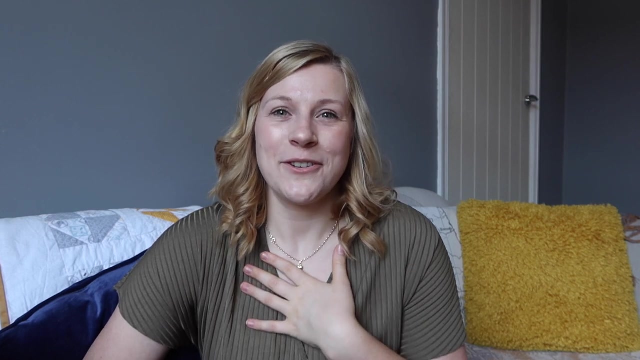 be able to get to the, get other sizes and if you are interested, and I'll leave all the links to everything in the description below. the dress is really cute and it's very inspired by Audrey Hepburn. the pictures are to die for. so you'll just fall in love with, like I did, because it just looks so adorable and so. 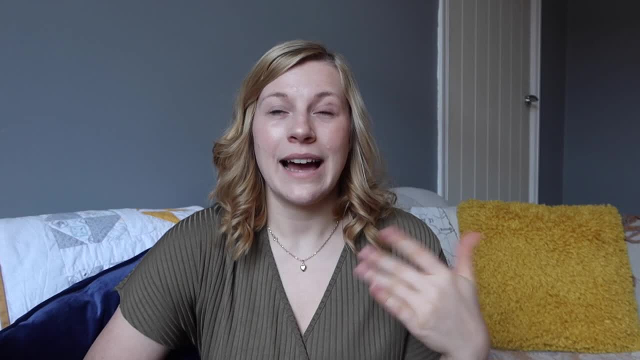 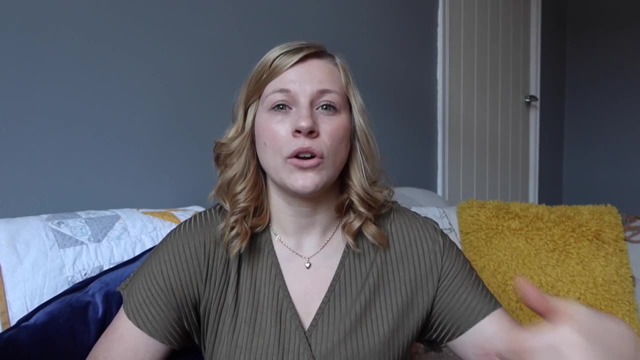 cute, but it is a little bit more advanced. so if you're looking for a bit of a challenge- and this is definitely something for you, if you are a beginner- I'd maybe look at doing some of the other ones first and then going back to this one later, when you've built up your confidence. so number nine on the list is 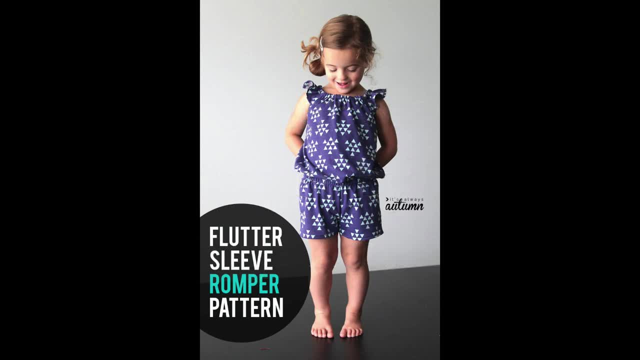 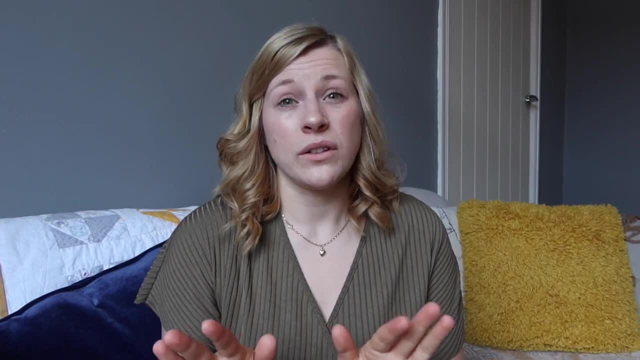 the flutter sleeve romper, but it's always autumn. this again is another super cute pattern and it's really adorable, and I would use this for boys or girls and just new, maybe change the sleeves and that's it, so I'll see you in the next video. bye, bye. 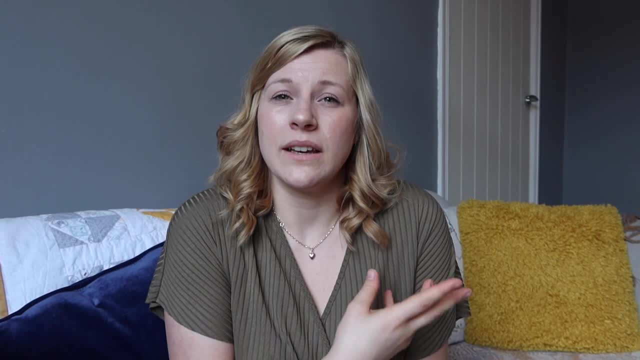 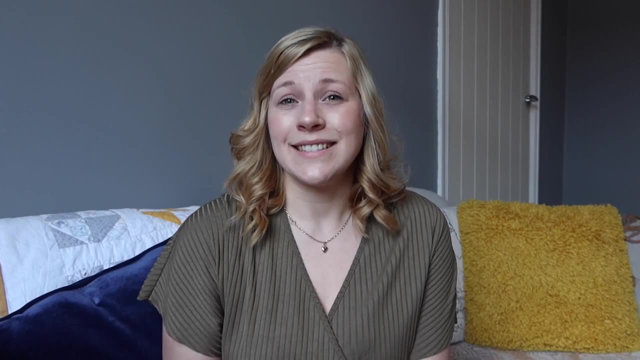 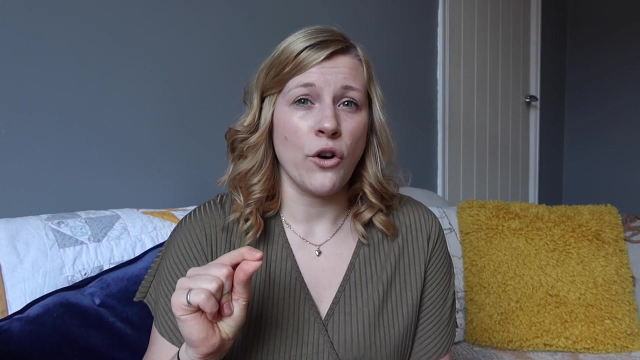 for boys. so it's, you know, maybe a sleeve instead of the like ruffle- totally depends on how you feel and how you want to dress your children, but I think it's really versatile and really handy to use. it's perfect for making a little summer holiday wardrobe and the size is restricted to 40. so that is an American. 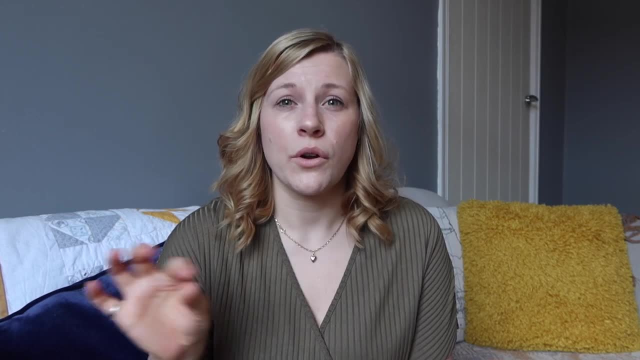 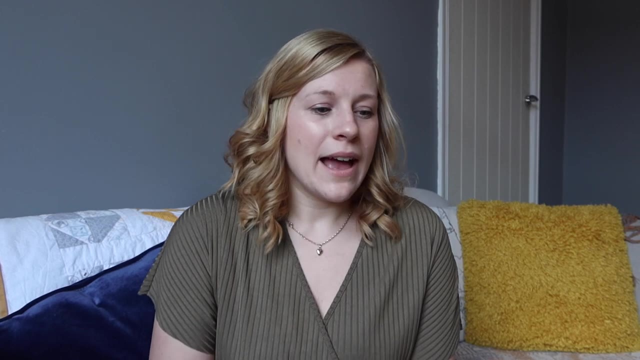 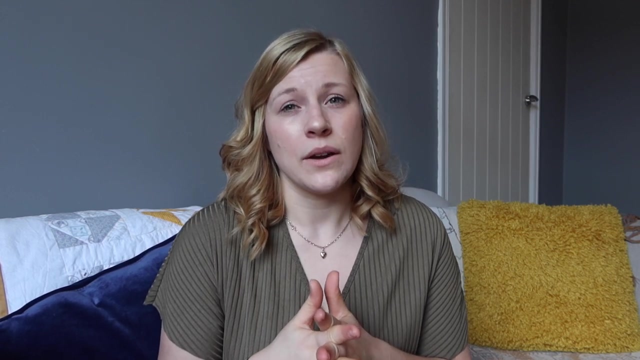 size and I'll obviously leave the information below from the conversions from UK, Europe and America sizes so you can work out if it's the right size for your child and but otherwise the pattern is really cute, really handy and quite simple to put together. it's definitely something that would make a 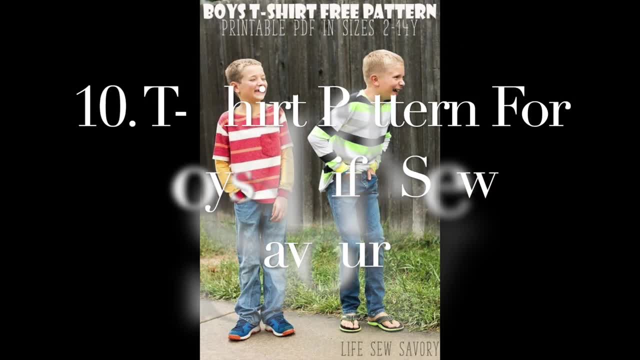 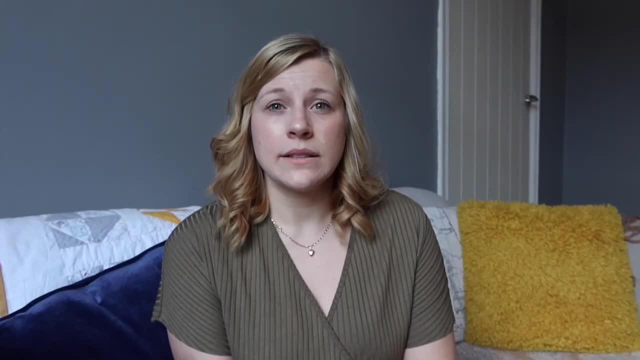 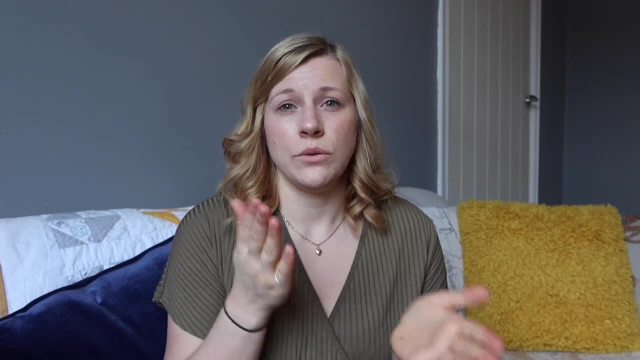 lovely little summer outfit. so number 10 is a t-shirt pattern for boys. by life, so savory this is. so this pattern is the is cut in the range of two ages, 2 to 14. so if you've got children between those years, that's perfect, because then you. 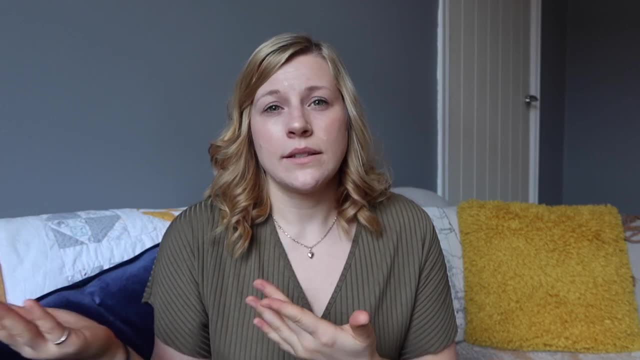 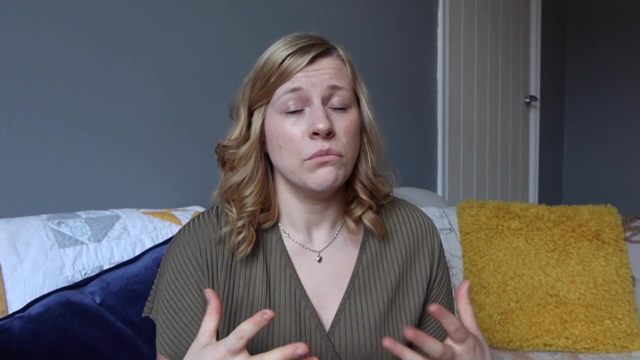 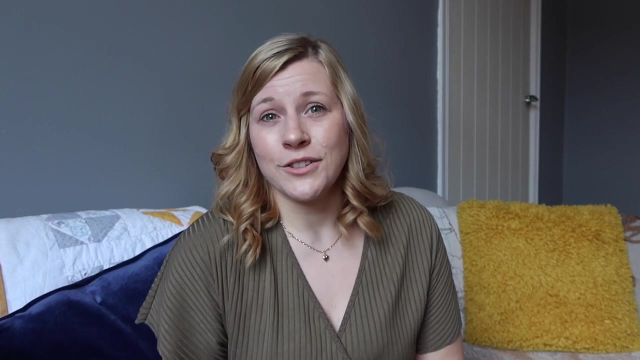 can use this pattern going up throughout the years to fit to them, their age, as they grow, which I really love because this is versatile. you're really getting a lot for no money at all. it's free, so you're getting a lot for nothing, which I really appreciate. um, so I think that is great. pattern's really simple to follow. the t-shirt. 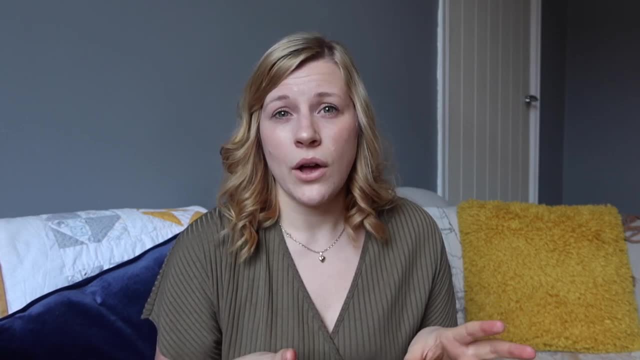 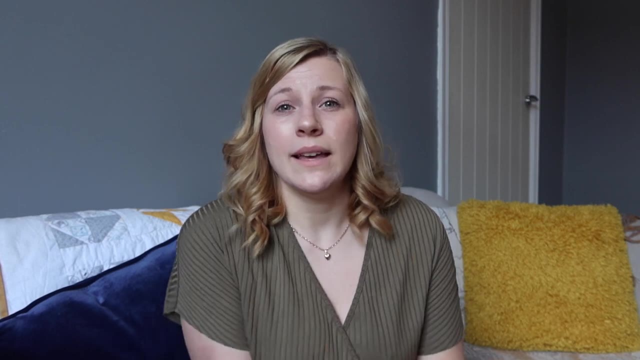 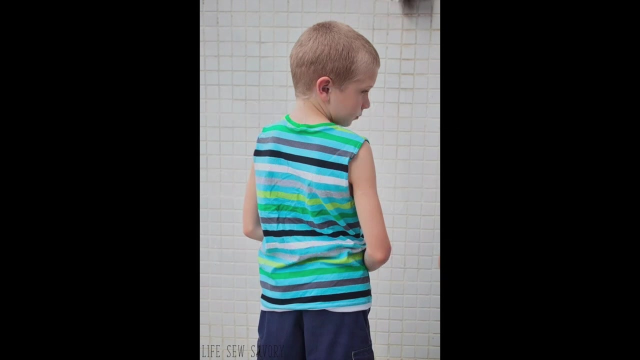 itself. they all look really beautiful. the pictures on her blog look so beautiful. so it's definitely something very inspiring and you know, it's really simple. you can make it within a day. number 11 on the list is a basic tank top, and this is again by life, so savory. so she has two boys and 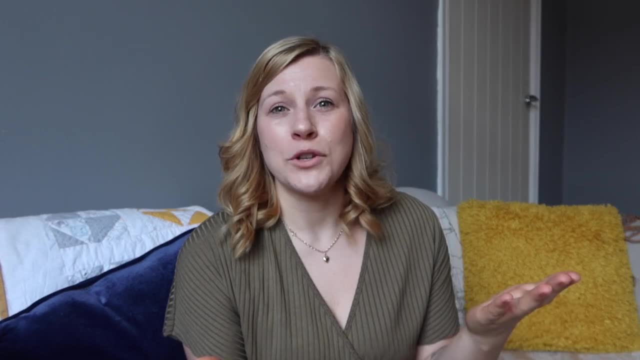 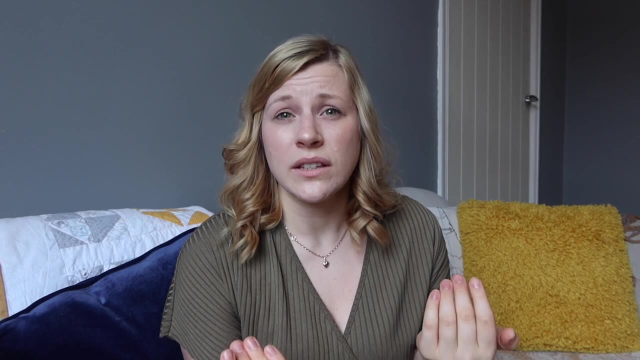 she's created these sewing patterns and again, the age range is from two years to 14 years, so it's perfect if you have children in that size. I would also say you could use this for girls, if you like, because it is so basic. you can just change up the fabric to be a bit more feminine, if you like. 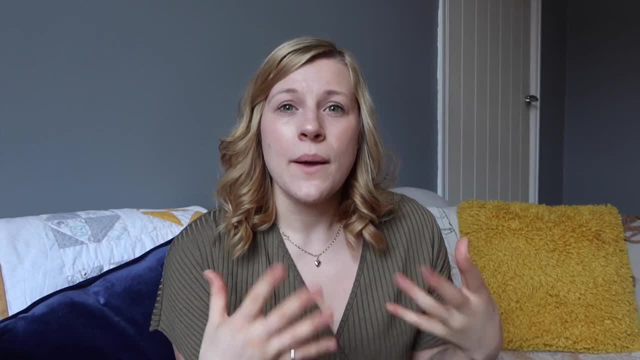 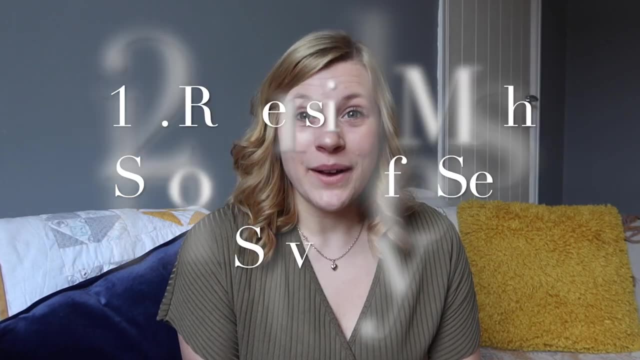 um, you can screen print on it. you know all these different things, but the, the actual template and the pattern is very basic, so you can use it for any kind of gender. number 12 on the list is some reversible mesh shorts, and this is again by life. so savory, she's definitely got you covered. 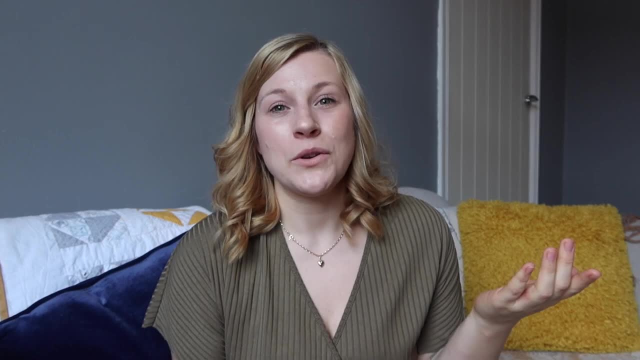 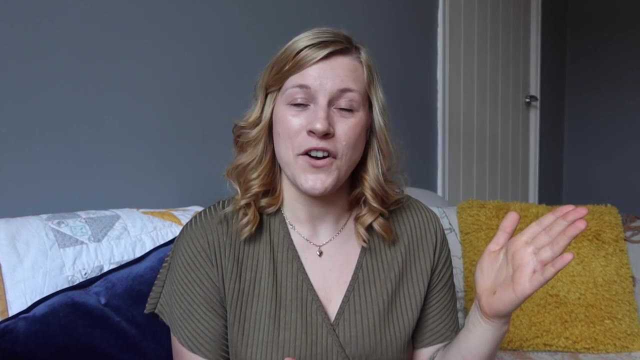 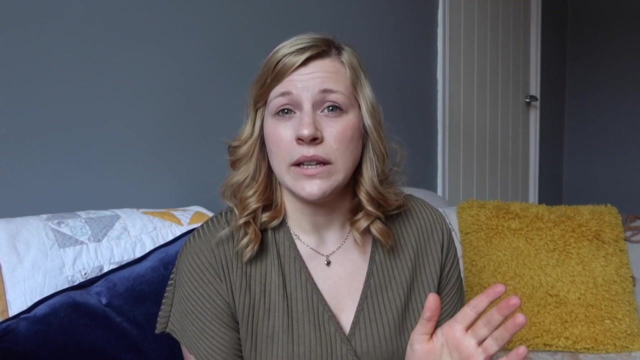 on these same patterns again. the age range is from two years to 14 years, so you know it's perfect because you can team these shorts up with a vest or a t-shirt from before and you've got a perfect summer wardrobe right there. so these shorts are really simple to put together. everything you need. 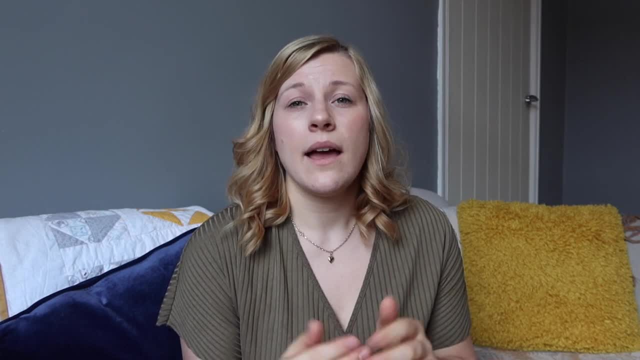 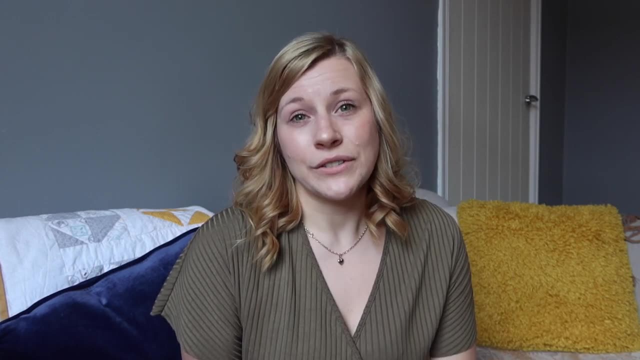 to know is provided for you within the blog post and the pattern, and really simple and really easy. and again, you can use this pattern again and again and again as your children grow. i would also say these make great shorts for sports activities because they're lightweight and loose, so even if 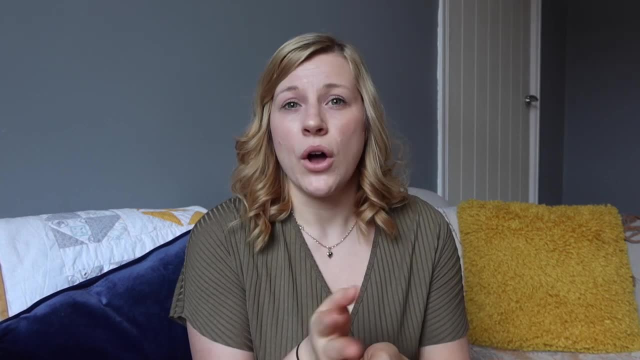 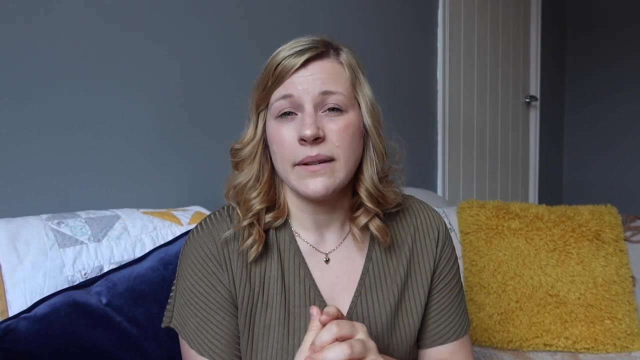 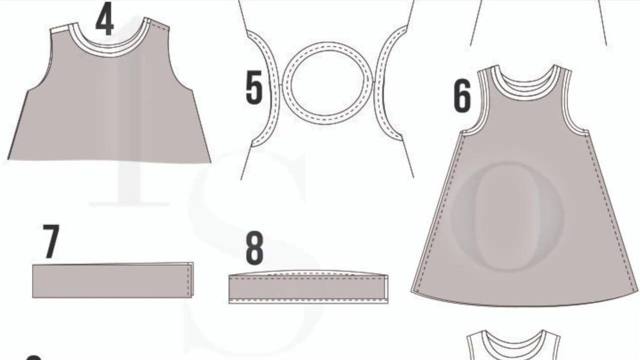 you've got girls that like to play soccer, football, tennis. you know all these different sports. perfect for pk. it's, it's, it's. you make your own, um, all things like that, just perfect. they're easy to put together and really quick. number 13 on our list is the summer 90 pattern. by so much ado, this is a limited age again. 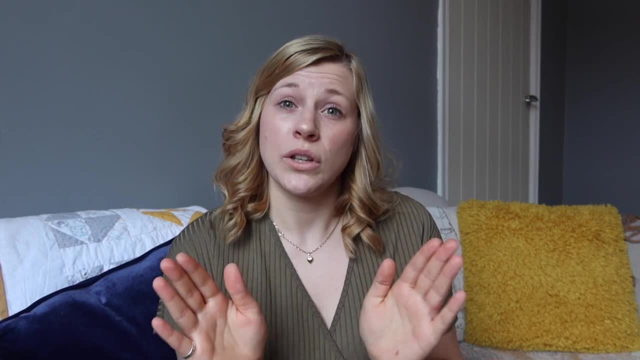 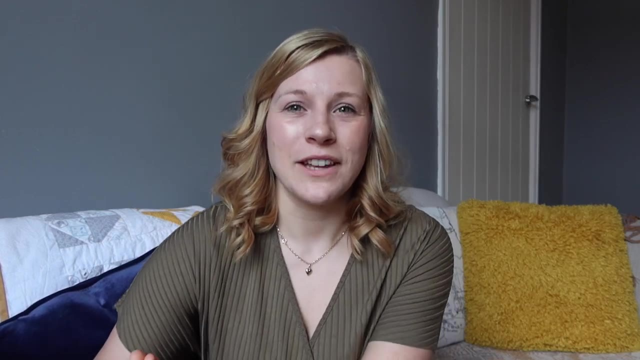 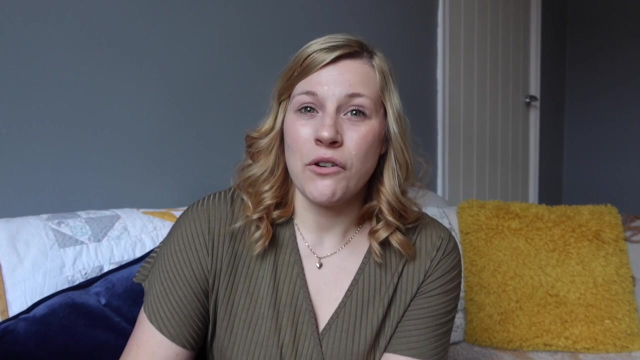 this is for two years to three years and it's a toddler range, um, and, but it is adorable. if you have children within that age range, then you definitely will want to make this. it's very cute and very feminine, very girly, um, it's very adorable. so, but i think if you have a child, that's just out. 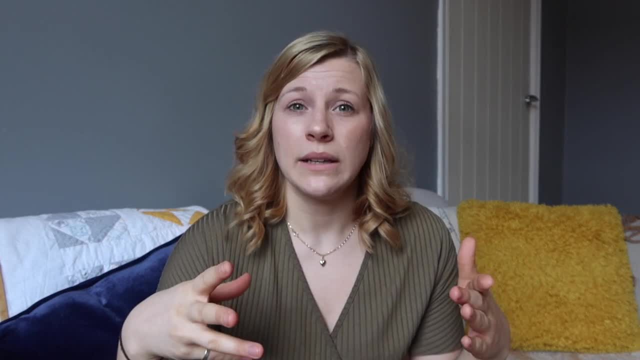 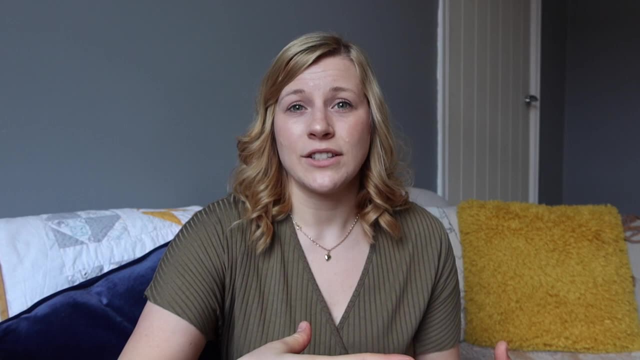 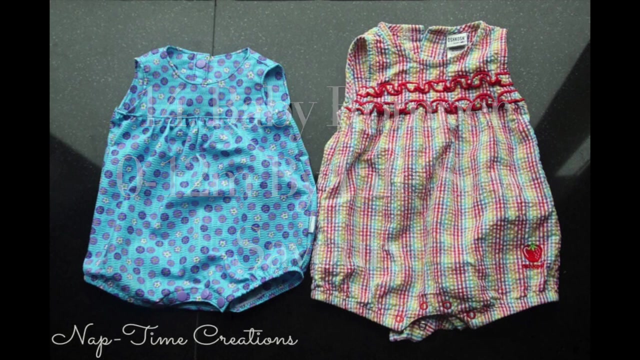 of that age range. you could easily use this pattern, just size it up a little to fit their needs and it's really simple to put together, really straightforward. but the after effect of the part of the actual garment is really nice. and finally, number 14 on our list is the baby romper. 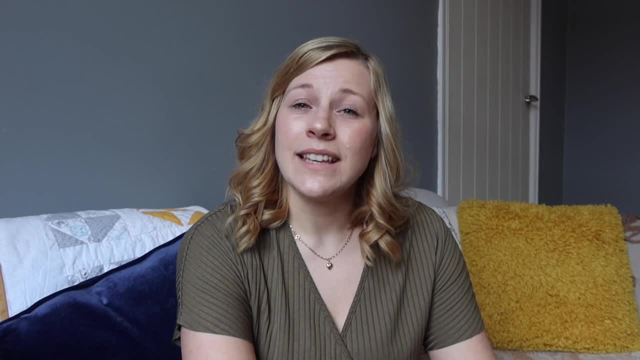 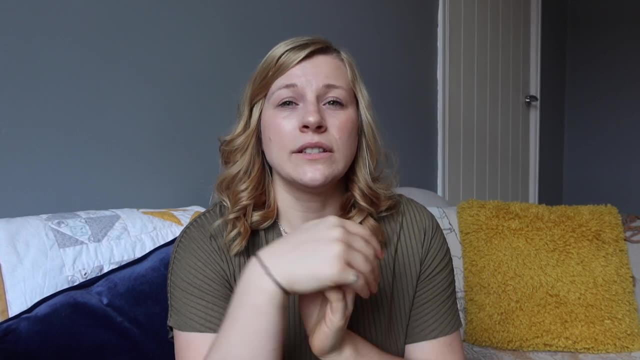 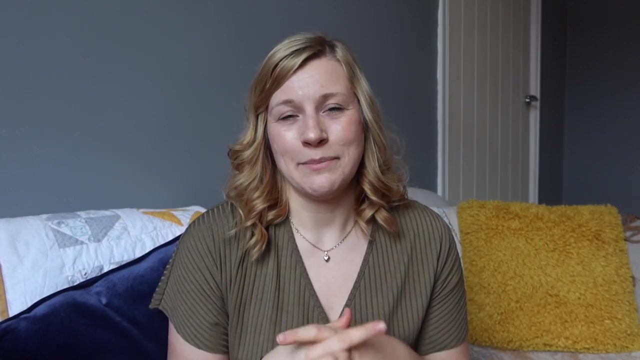 not 12 months by life. so savory. this is adorable. it is so cute. you can make this up for a friend, for yourself, for you know somebody that you know that's having a baby. it makes a perfect gift and what's more is that it's homemade and made with. 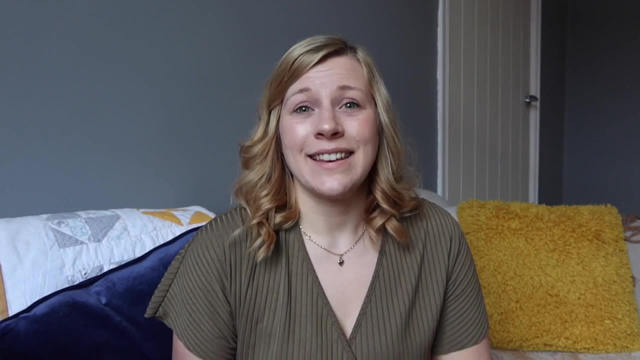 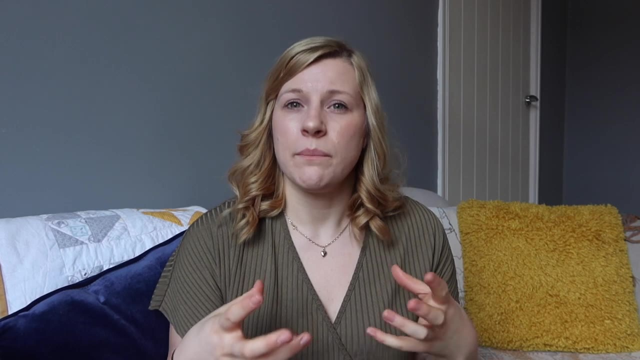 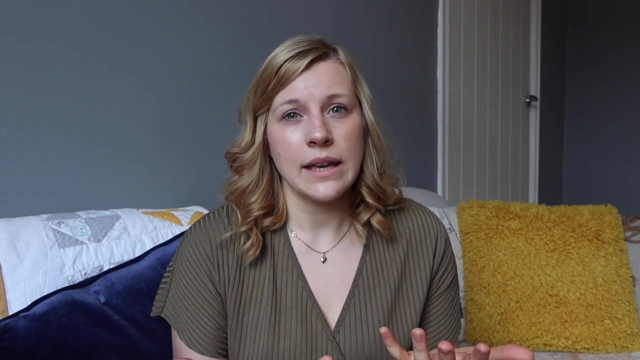 love by you, which i i really love. i think it's adorable and it's really simple to put together, really easy to follow. i think rompers and baby clothing can often be quite daunting to get into, but you know the blog and the, the lady that created these. she talks about it in such a way that it's so easy to understand.